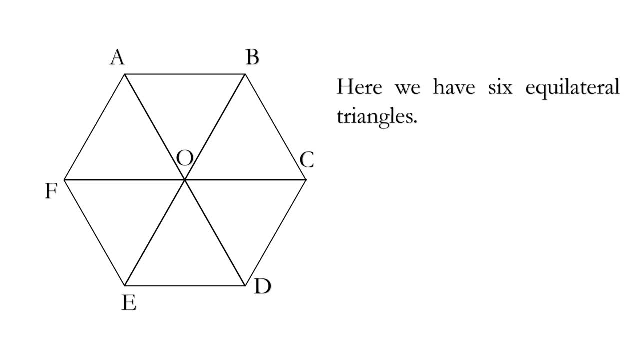 longer diagonals, We can see that it consists six equilateral triangles. So therefore, in this figure, AB is equal to OF, is equal to OC. Hence we can conclude that its longer diagonals are twice the size. Now let's draw a shorter diagonal, BD. Here we know that if the side length is A, 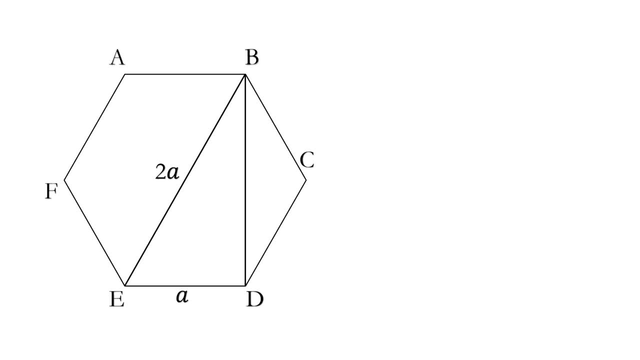 then longer diagonal must be twice the A, that is 2A. Now in this right angled triangle we can apply Pythagoras and conclude that its shorter diagonal is root 3 times the side. We will use these two conclusions for the renewal in this example. 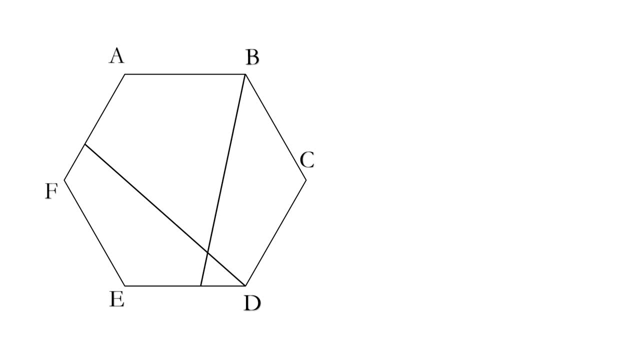 Now use theikk's formula 1.. Here let's draw the figure in this arrow: 2023. as in the question, Let's name these Q points, sg and aku. So we will divide these by 2 ag here into complex and complex. 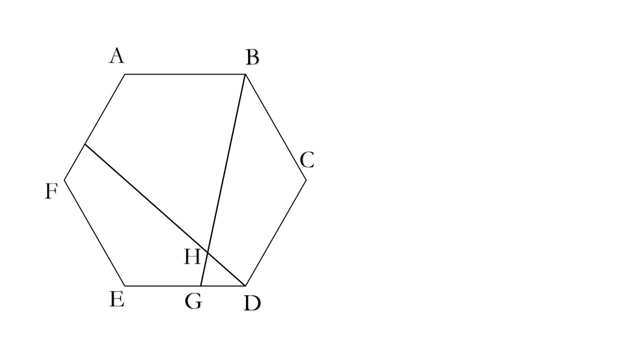 Let's name these points as g, ialsvs, Its leader, U, 5, h. here we have drawn one of the smaller angles, that is, one of the yellow regions. draw BD and suppose the angle GBD is theta side length. AB is 3 here as given. 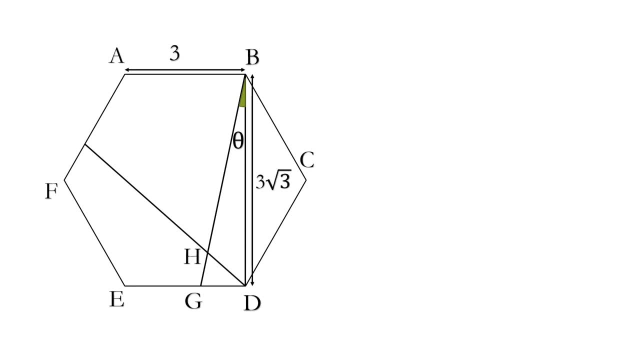 in the question. so from our second conclusion we can write: BD is equal to 3 root 3 because shorter Eisenhower three times beside. now in triangle GBD we get 10. theta is equal to 1 over 3 root 3. with this data we can calculate: 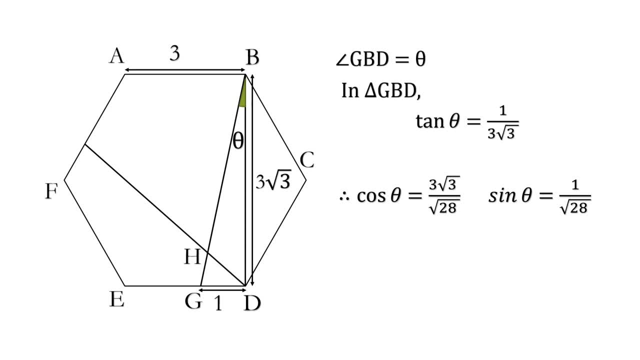 cos theta and sine theta easily. so we get: cos theta is equal to 3 root 3, reporting to 20, min insane criticize. equal to one over root 20, since the figure is symmetric from all the sides. hence the angle GHB in each yellow triangle must be equal, and if the angle is equal, so it must be 60 degree. 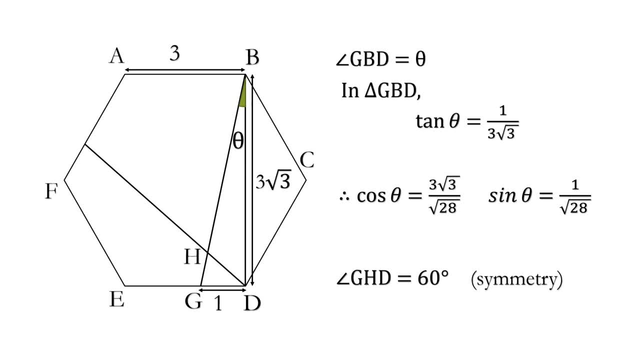 because if it exceeds 60 degree, then the complete rotation will not be 360 degree, it will exceed 360 degree. hence the angle GHD must be 60 degrees. in triangle GBT, angle HGD is equal to 90 degree minus theta, because it's the right. 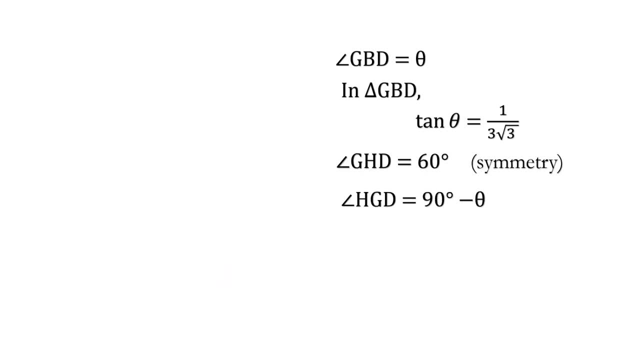 triangle. for a while we will focus only on this smaller triangle, the yellow region. so here this is the triangle for which we have to calculate the area. okay, also, we can write: angle HDG is equal to 180 degree minus the sum of other two angles and we get angle HDG is equal to 30 degrees plus theta. if in a triangle, 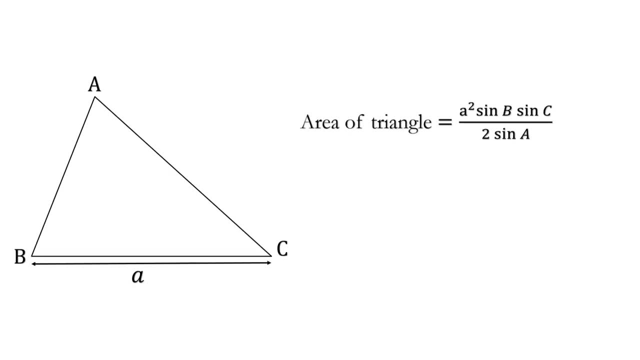 two base angles are given and the length of base is given, then we can apply the formula a square sine B, sine C over 2 a to calculate its area. okay, so we will apply the same formula here and we get: the area of triangle is equal to cos theta. 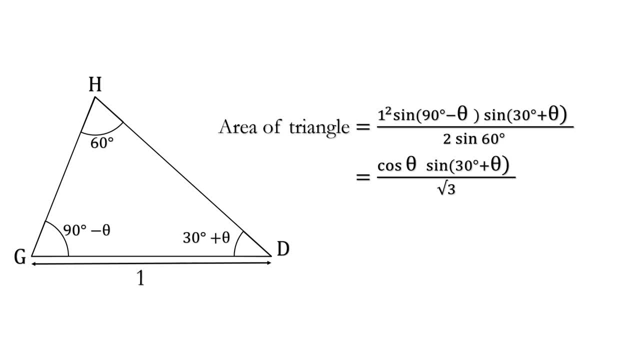 sine 30 plus theta over root 3. on expanding the sine 30 degree plus theta we get: area of triangle is equal to 3 root 3 over root 3 root 28 in bracket 1 by 2: 3 root 3 over root 28 plus root 3 over 2 multiplied by 1 over root 28. 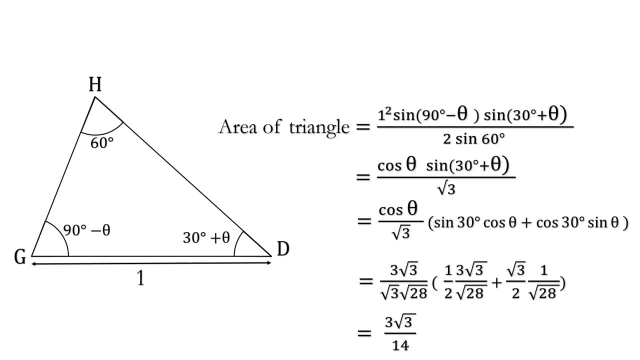 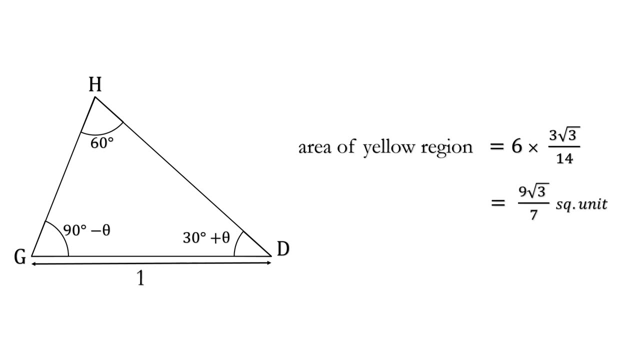 and on simplification we have: area of the triangle is equal to 3 root 3 over 14, since yellow region consists six these triangles. so area of yellow region is equal to 9 root 3 over 7 square units. now let's come to the figure. 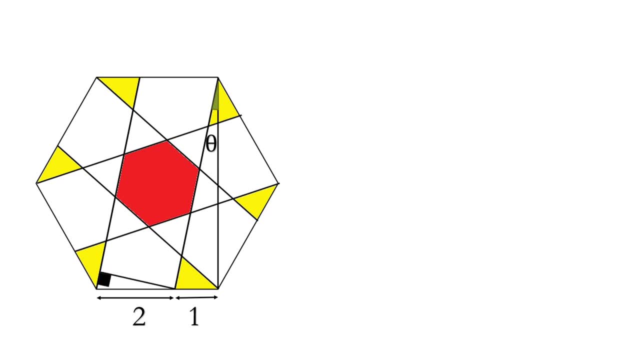 draw a perpendicular, something like this. in this figure the angle here shown is theta, because these two sides are at a right angle from each other. also, one of the sides is making a angle of night theta from another side. so if we draw our side perpendicular this another side, then the angle between these two also be theta or. 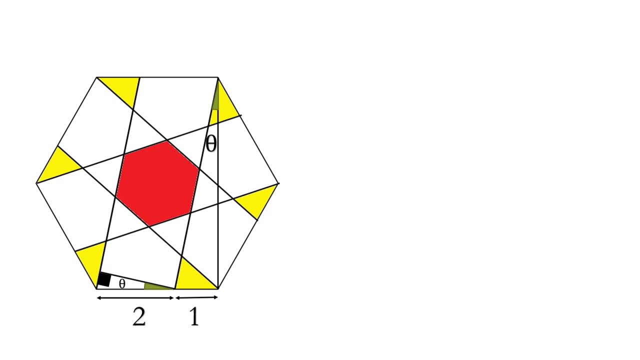 theta is equal to this angle we get for this type of平th. we can get that here. so from the second glass here we can get. for red hexagon, length of the shorter diagonal is two cos. theta ie 2 multiply by 3 root 3 over 28.. 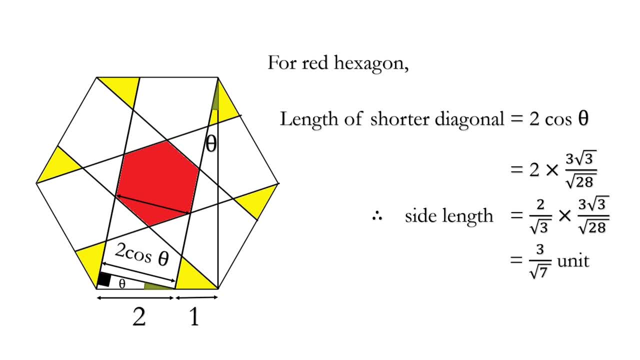 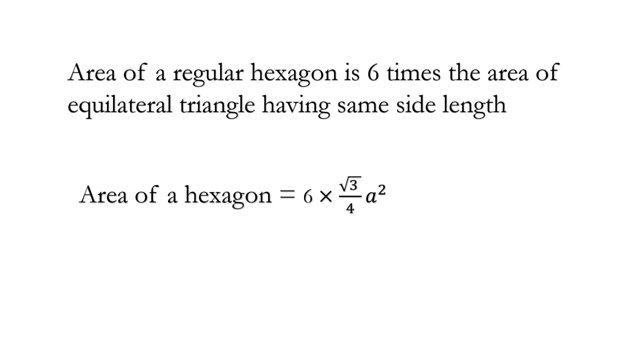 root 3 times this shorter diagonal, which is equal to 3 over root 7 units. Now, area of a regular hexagon is 6 times the area of equilateral triangle having same side, because it consists 6 such triangles. Therefore, area of hexagon is equal to 3 root 3 over 2a square, where a is the side of the. 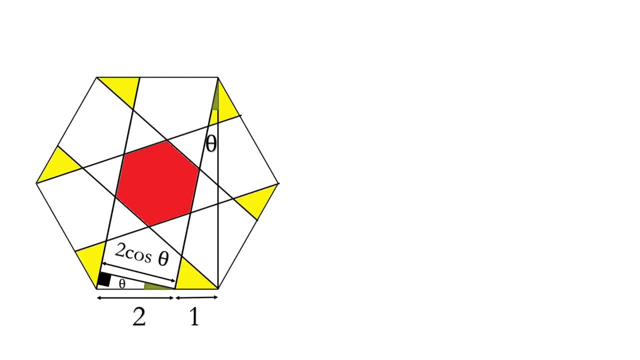 regular hexagon. Therefore, the area of red region must be equal to the area of this hexagon and we get 27 root 3 over 14 square units. Now ratio of red and yellow region is equal to 27 root 3 over 14. ratio 9 root 3 over 7. 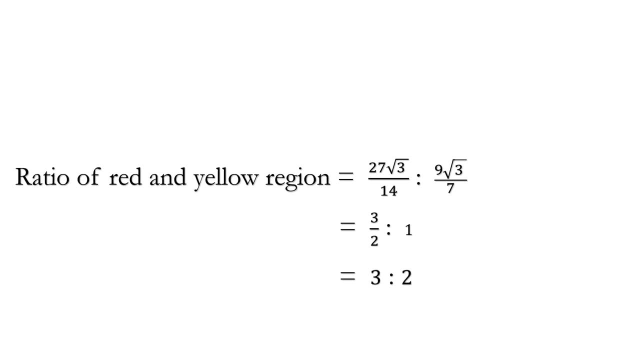 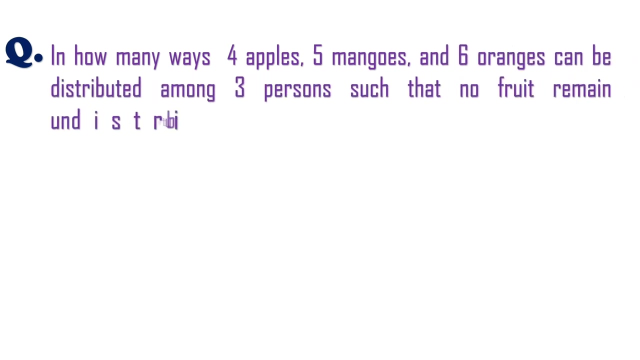 that is 3 by 2 ratio 1. And that is equal to 3 ratio 2, and this is our solution. Let's move to over another question: In how many ways 4 apples, 5 mangoes and 6 oranges can be distributed among 3 persons? 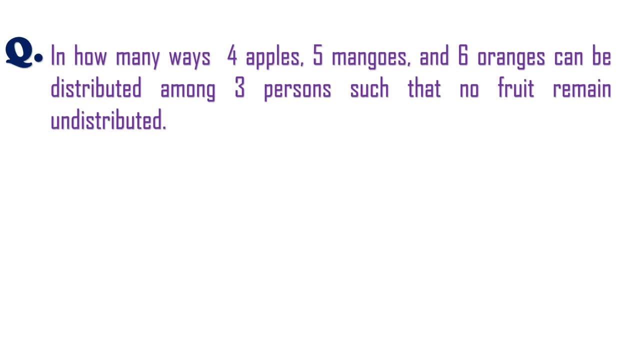 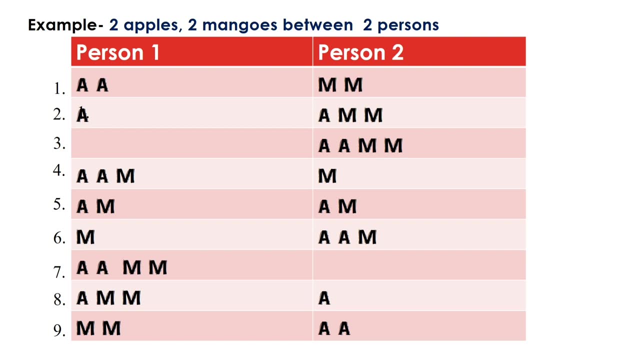 such that no fruit remain undistributed. For example, if 2 apples and 2 mangoes are distributed between 2 persons, then here all such fruits are distributed. All such combinations are given where a represents an apple and m represents a mango, and you have to do the same thing for our question. 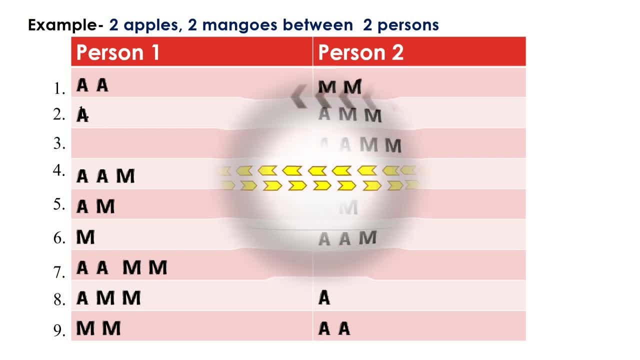 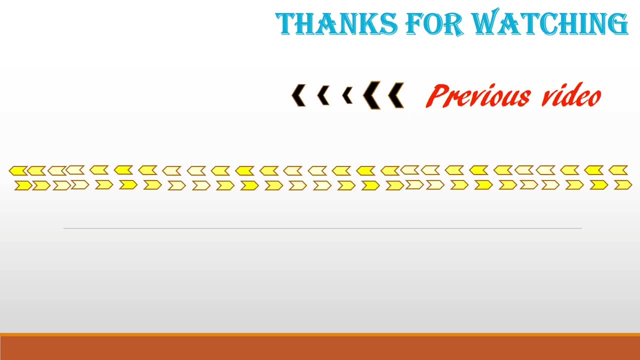 Try this question and comment us the solution, and if you have any question like this, send us on the gmail given in the description box. If your answer is correct, we will announce your name in our next video. Don't forget to like and share our video and for more such videos, subscribe to our channel. Brain Exploders. Thanks for watching.